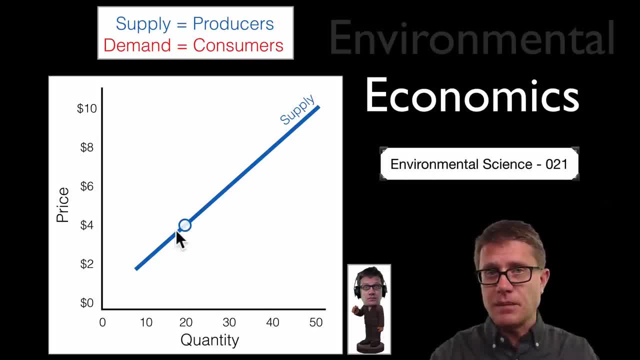 that is going to be right here on the supply curve. I do not want to invest a lot of money. I am not going to make a lot of profit. I do not make many. Now there is also going to be a demand curve. This is how much they want it, And so if it is really cheap, they. 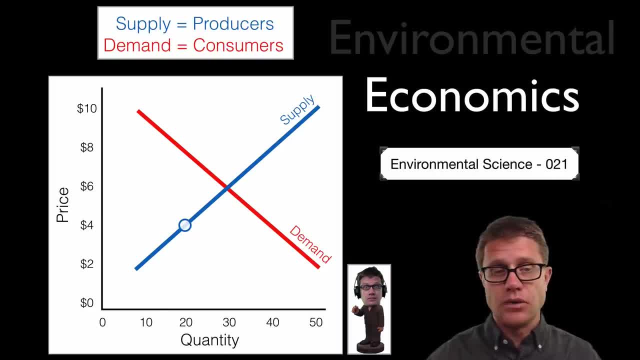 want a lot of them. If it is really expensive. they do not want very many, And so if we play this across at $4, we find that their demand. they demand 40 of them. I have only made 20 of them. And so what do we get? We get a shortage. I did not make enough of them. Now I know. 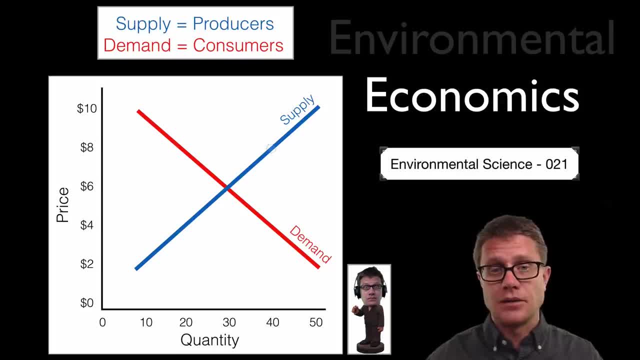 a little bit more. So people want them. There is demand, it looks like. So I am going to go all in, I am going to spend a bunch of money, I am going to make a lot of them And I am going to charge a lot of money, hoping to get a lot of profit. And so if I charge, 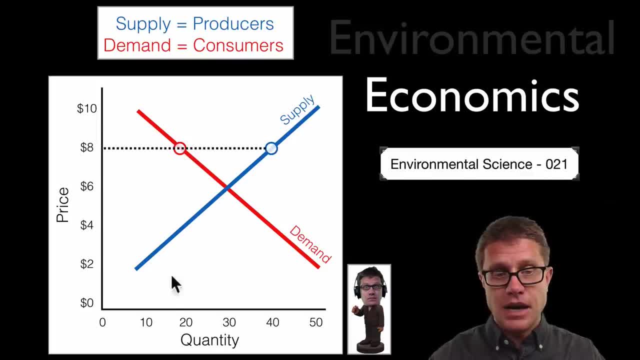 $8,. watch what has happened to me, What has happened to the demand. Now the demand is 20.. But I have made 40. And so what do I have at this point? We have got a surplus, We have too many of them, And so you can figure. 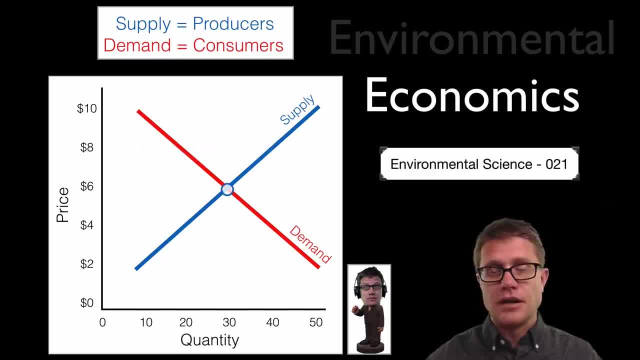 out where I am headed here. What do I want to do is I want to make sure that I hit right where those lines cross. Again, there is no graph like this. This is just trial and error. But you want to hit what is called equilibrium where the price hits the demand. That is economics. 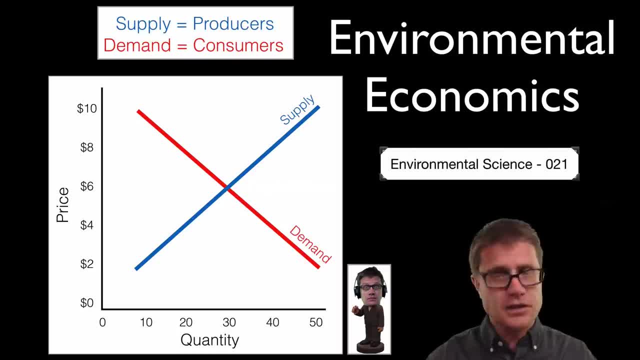 Now, what is environmental economics, though? It says law of supply and demand is right, But what you are not including are the externalities. In other words, to make a bobble head, it is way too cheap. It is cheap because you are using maybe cheap labor. You are making it. 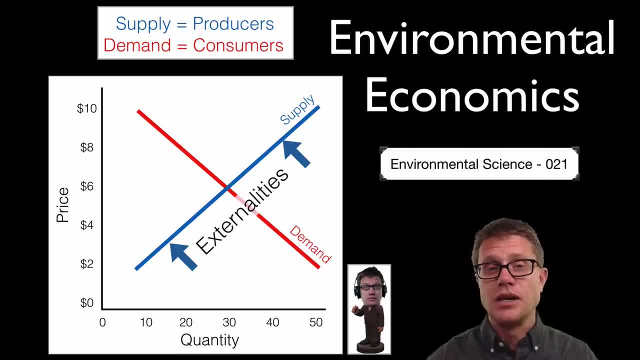 in a developing country. Maybe you are polluting the atmosphere, So you are really. your price curve or your supply curve should be pushed in that direction. So if we push it in that direction, what does that mean? We are going to have a new equilibrium at this point In. 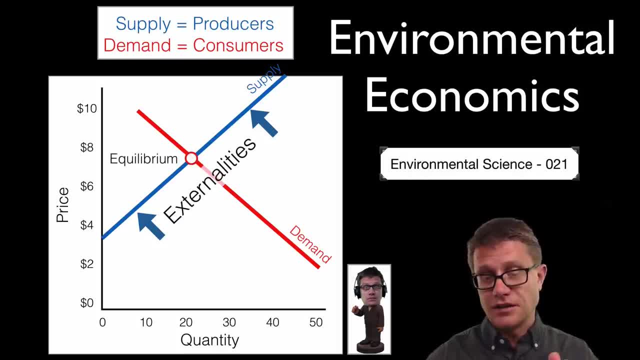 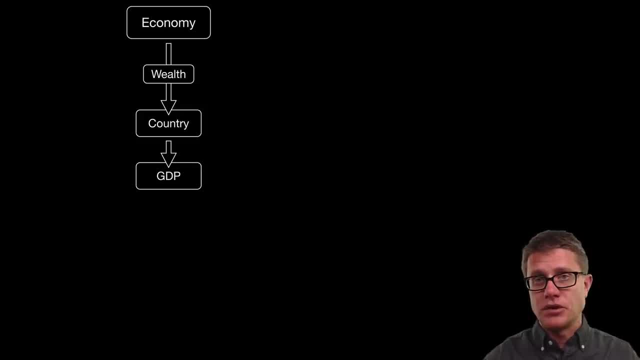 other words, things are going to cost more if we pay for externalities and people are going to have less, And so the economy is really the wealth of a country, And a good way to measure that is through the GDP or the gross domestic product. Now, the decisions that we make are governed. 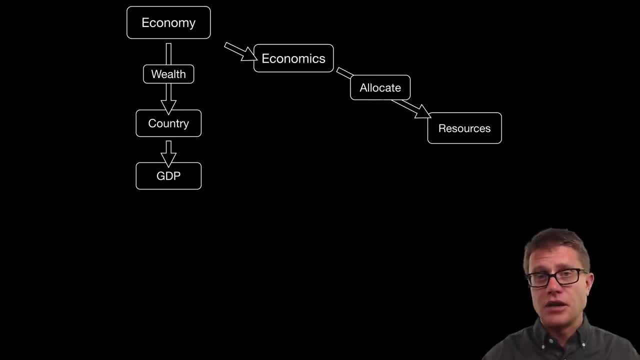 by economics. What we are really trying to do is allocate scarce resources, And we are using those resources through production, making things, consuming them and then moving them around, So that law of supply and demand applies at this point. Now the problem is: 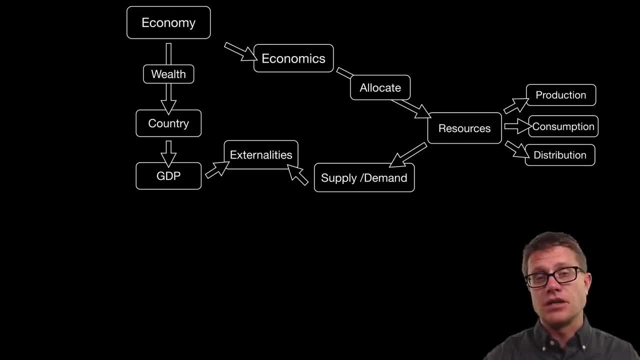 that GDP and supply and demand both do not take into consideration these externalities. Those are the costs to the environment and ecosystem services, And a lot of the time, what we end up with, for example, if we are looking at the atmosphere, is pollution. We 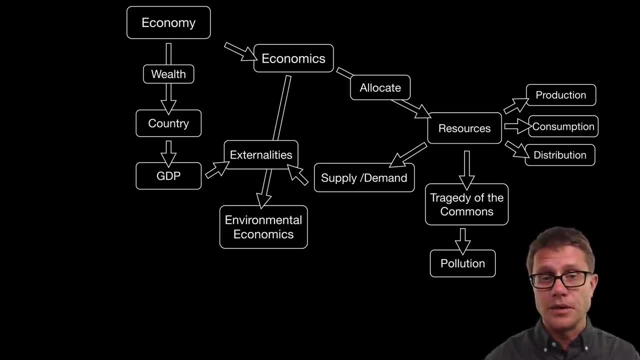 are increasing carbon dioxide levels, It is leading to global warming, And so a lot of people are putting this forward. This idea of economics is at the center. That is going to have our solution, So let's move towards environmental economics. If you just let the 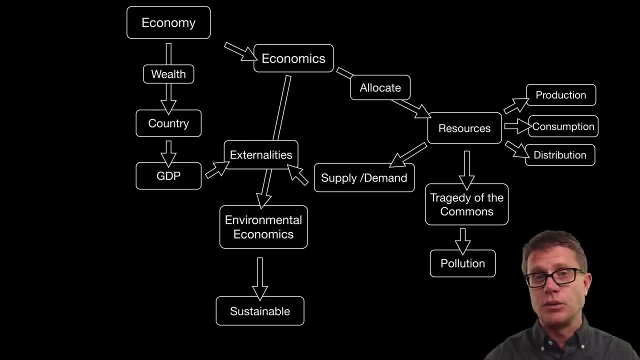 market go. it is not going to solve this problem. We need a sustainable system. First thing we have to do was replace the GDP. A good alternative would very much be the interocupational E fazem miracles and change the economy. I think that is really smart. I have heard much talk about that, But if you are looking 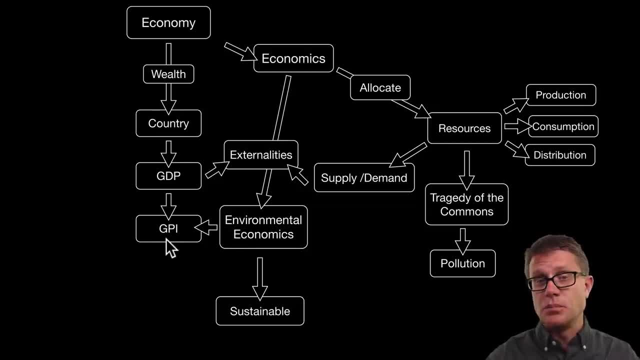 not to change the economy. we can't change the economy. At the very least, a lot of the questions- and I think a lot of these questions are based on the water generated from. the alternative would be the GPI or the Genuine Progress Index. that includes these externalities. 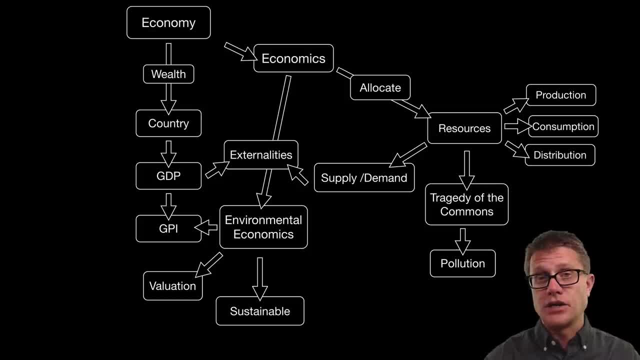 into the wealth of a nation. We could also add valuation. So give value to these ecosystem services, And then we may have to do some regulation to decrease the amount of pollution. An example put forward is this idea of caps. So we are capping the amount of pollution. 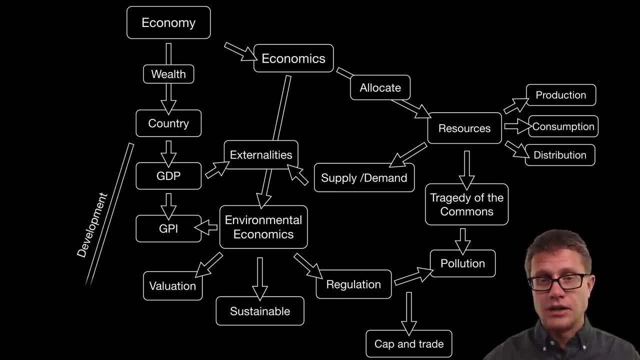 that you have And then allowing some of those caps to be traded. There is some controversy there, But the key point is to understand that we are a highly developed nation And that other countries are developing And there is something called the Kuznets curve And 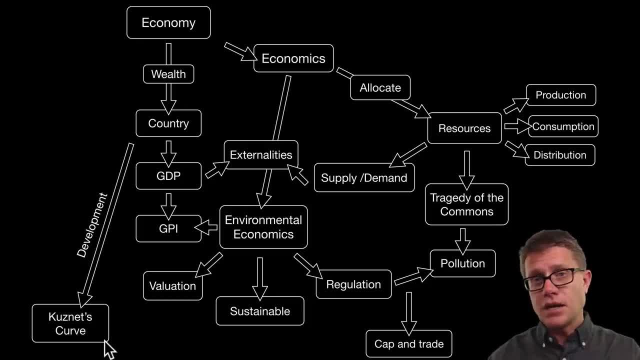 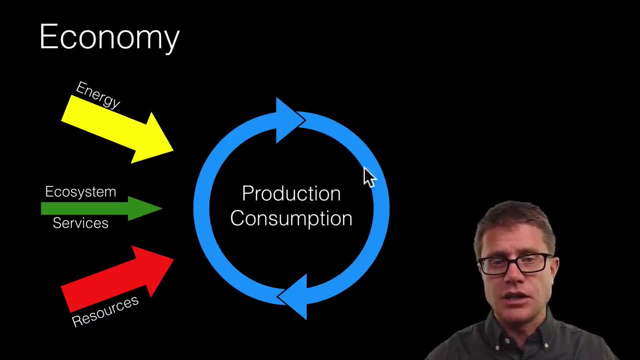 this idea that until your country is wealthy enough to think about the environment and environmental economics, you simply will not. And so if we think of the economy like this, it is production and consumption, So we are taking in energy, using ecosystem services and using resources, And so this we can think of as a slow economy. It is not consuming. 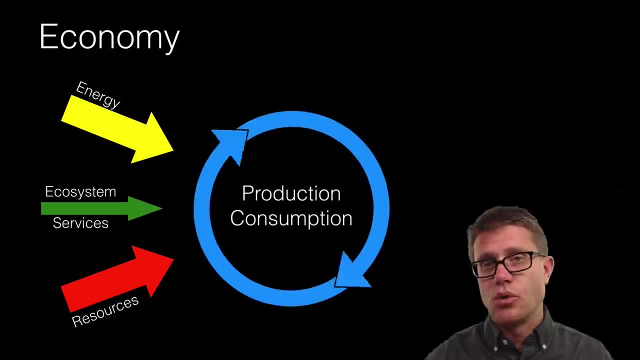 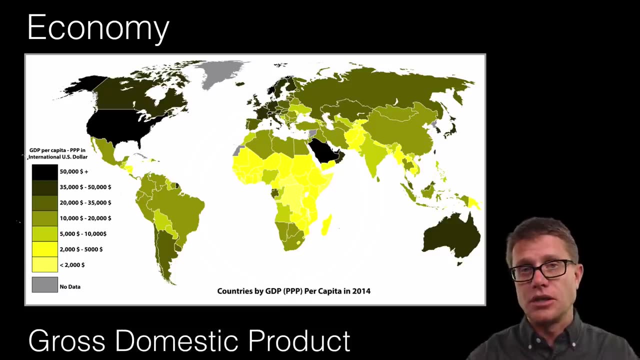 much. This would be an economy that is consuming more energy, more resources, And so a good measure of that is going to be the gross domestic product. How many things are you producing and therefore consuming? And so, if we look at it, in the US, the GDP is over $50,000. 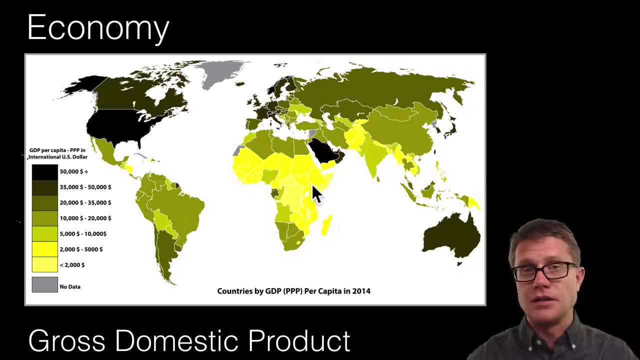 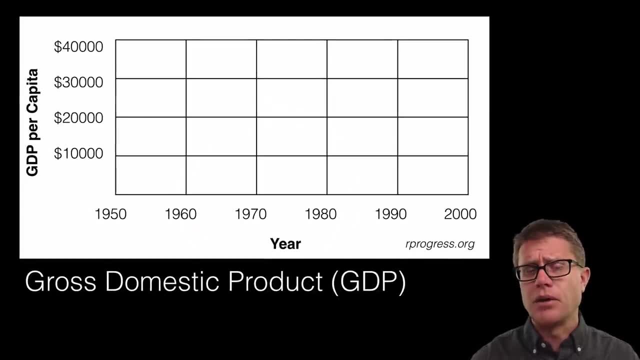 per person, But there are going to be certain areas where that number is going to be less than 2,000.. So we see that same thing of developing versus developed nations. If we look at, however, the world over time from 1950 to 2000,, you 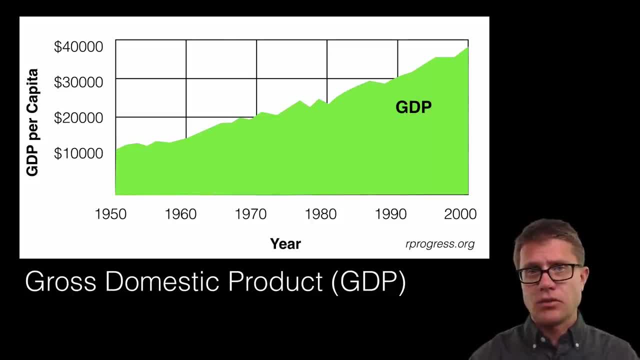 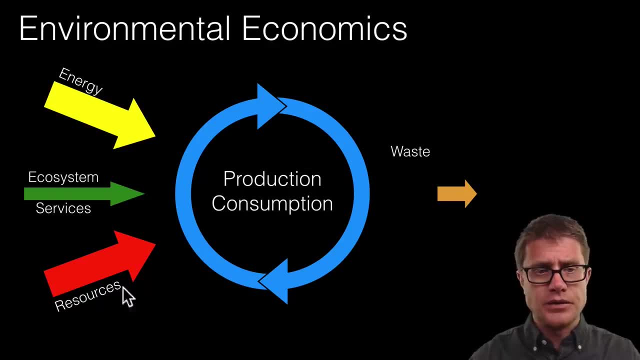 can see that the GDP keeps going up, And so you might think: well, this is great, So countries are getting wealthier, We do not have anything to worry about. But my model was inefficient, So what I had included was the inputs, but not the outputs. And so what? 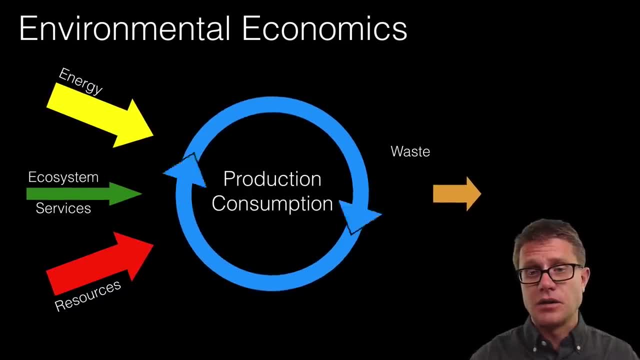 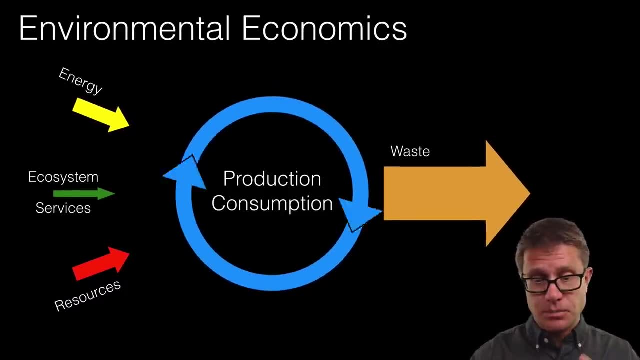 we are really not dealing with is waste. And so, as the economy turns, watch what happens to the waste. We deplete the inputs and we increase the outputs. There is pollution, health concerns. As the economy goes faster, waste becomes a bigger deal. What does that? mean. So if you look at the different kinds of goods we have in this economy In general, all of these products we have here are going to be water-based, So we are going to see that our emissions in the US are going to be more. This is why we are going to have to do something. 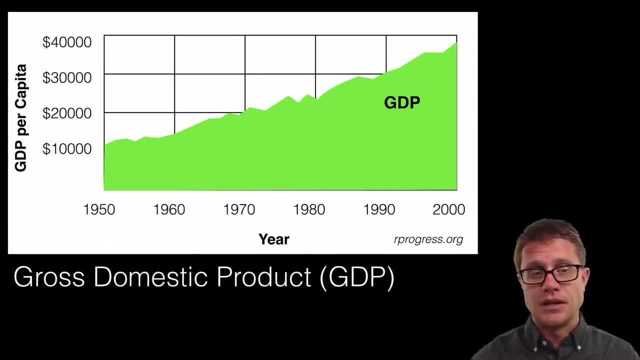 waste becomes a bigger deal, And so some people are putting forward this idea of replacing the gross domestic product with the GPI or the genuine progress index or indicator, And what that includes is not just how much money you are making, but pollution, resource depletion. 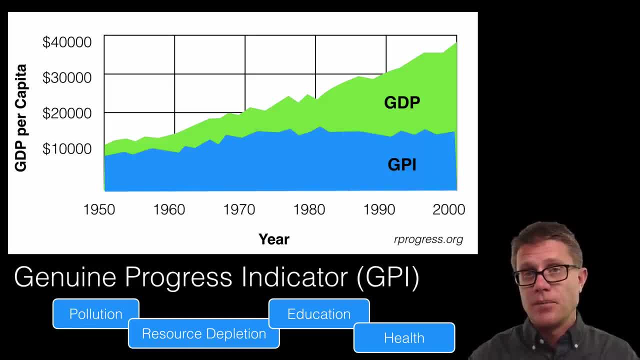 the health of the people, education of the people And, if we look at that, that across the world, according to this, our progress model has been flat lined for the last 40 years. That means that we are not advancing. So the market has only brought us so far, And so 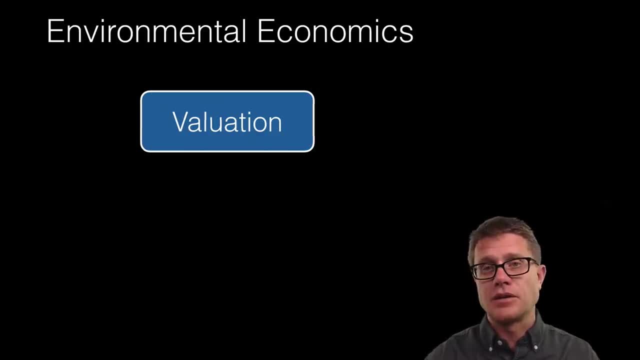 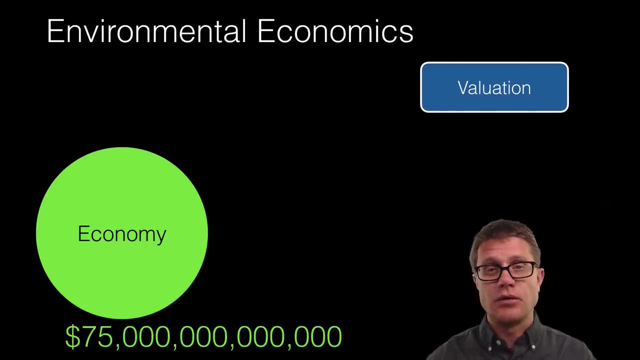 environmental economics is: how can we use the power of economics to solve this problem? The first one is the idea of valuation, And so if we look at the economy on our planet, it is $75 trillion. But remember, outside of that we have ecosystem services. Those are: 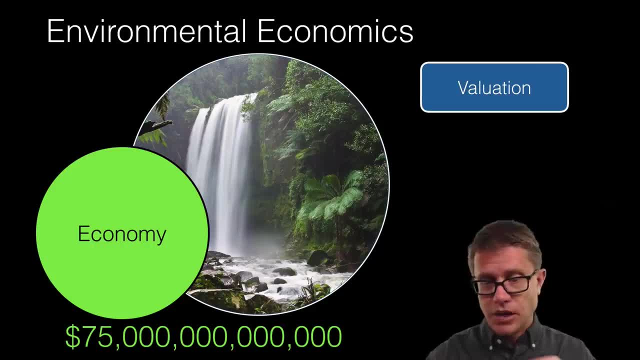 things that the planet is doing for free. So, for example, they are filtering our water, They are taking in carbon dioxide, They are providing energy, And so we do not pay anything for that. So we should add value. So we should add value to that. If there is no monetary value to it, people are not going. 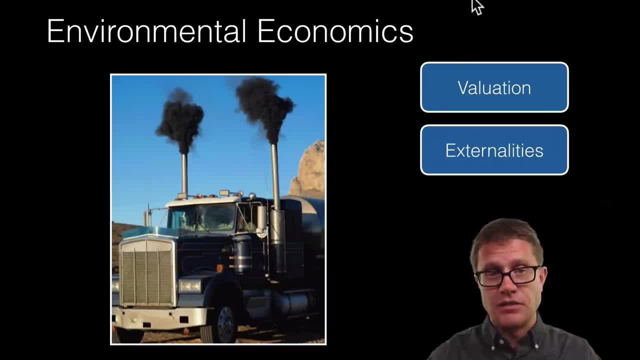 to see value in it. We also have to discuss the idea of externalities. This pollution coming out of this truck, the people in the truck are not paying for it. The people who are moving the material are not paying for that increased carbon dioxide and what that. 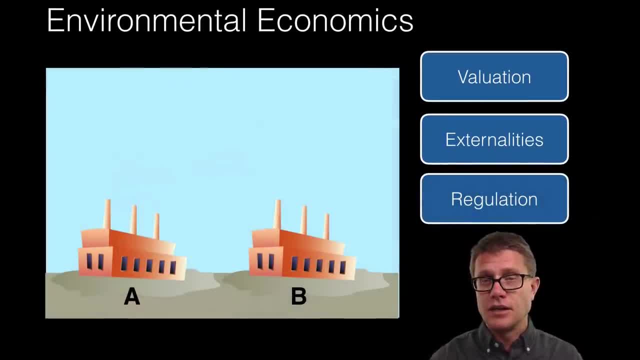 is doing to the planet And so we have to start discussing those externalities And it may lead to certain regulations. So if we are looking at two factories, factory A and B, and they both are polluting, So if we say they are polluting like that, they 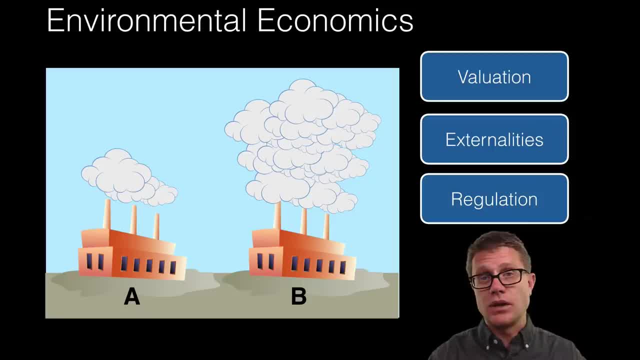 will be polluting those factories. We have to value that pollution. How much does it cost? What externalities do we have from that? And then we have to regulate it So we could set a cap. This is the amount that you can pollute. We call that a cap, And some people 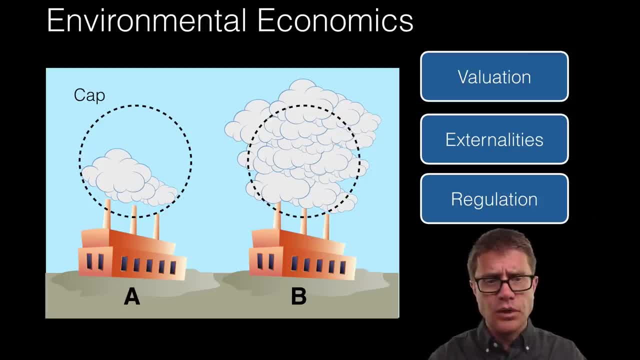 are putting forward this idea of cap and trade. What does that mean? Well, factory A is well within the cap, And you can see that factory B is way outside the cap. It is polluting too much, And so the idea is that you could trade some of those credits from factory A. 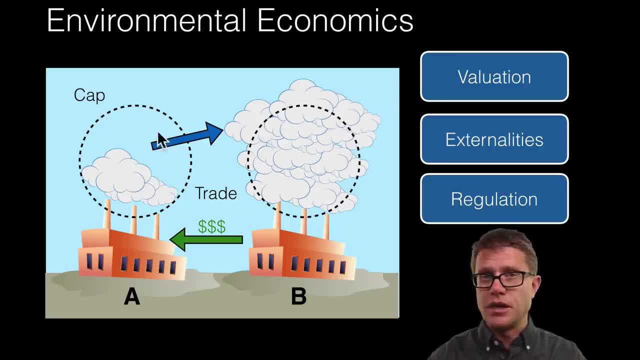 factory B, So you can keep polluting because it is essentially within this cap, And in return, you are going to pay me money. Now this is weird. We are creating these economics of pollution, But it has been pretty successful If we look back at the acid rain program, where 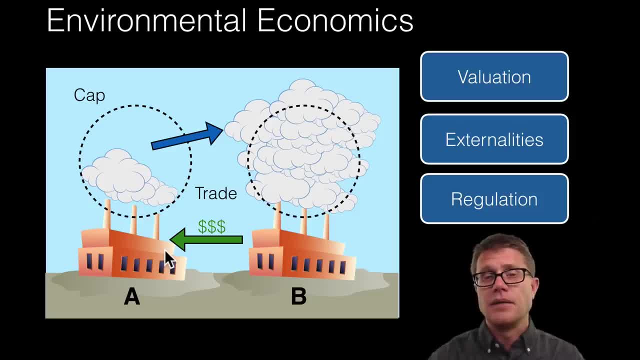 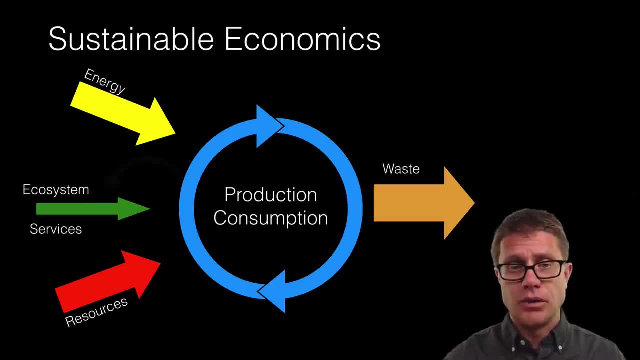 we were doing cap and trade with the amount of sulfur dioxide. it showed some increases, And so a better way to look at sustainable economics is a model like this. So what we want to do is take the power of that economy and return those ecosystem services and recycle. 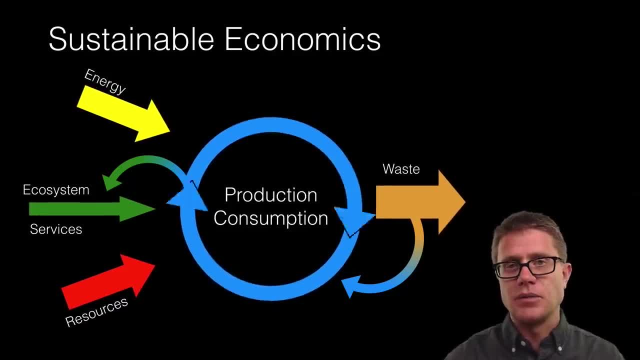 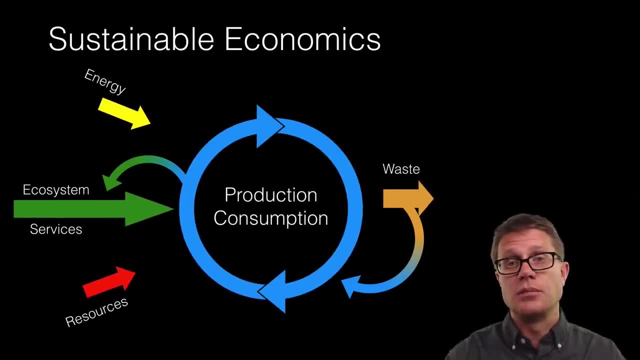 that waste, Because if we can have a sustainable system like this, we can decrease the amount of waste, And this is something that allows us to have increase in not only the GDP but the GPI as well. Now, what is the problem is that countries are all along the spectrum. 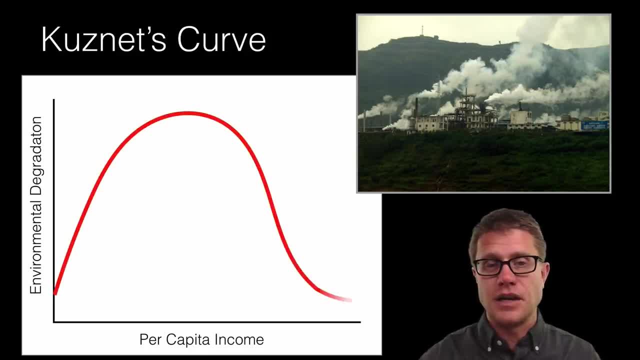 of development And there is the Kuznets curve And it kind of goes like this: It is this idea that as your economy is increasing, increasing, increasing, increasing, increasing, increasing income is going up, you will actually worsen the environment until you hit a point where, 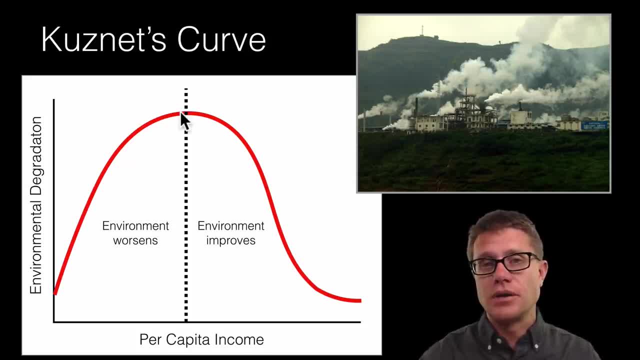 you can start to improve the environment. In other words, as a country is growing, they cannot spend money on these ecosystem services and they will not. And we also have problems with globalization now. So once we have a developed country with really strict regulations, we can move some of those factories to an area where they do not have such strict regulations.